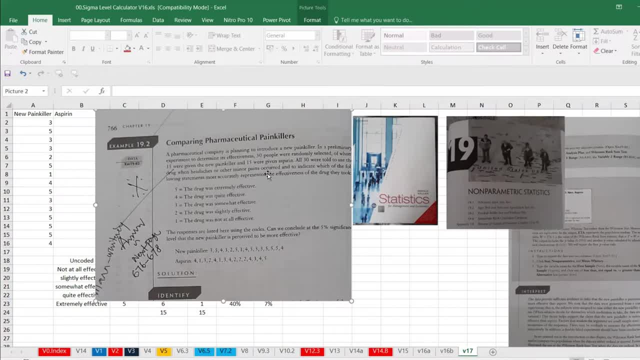 when headache or any other minor pains occurred, And to indicate which of the following statement most accurately represented the effectiveness of the drug they took. They have given five: that means the drug was extremely effective. Four: the drug, the medicine, was quite effective. Three: somewhat effective. Two: slightly effective. One: not at all. 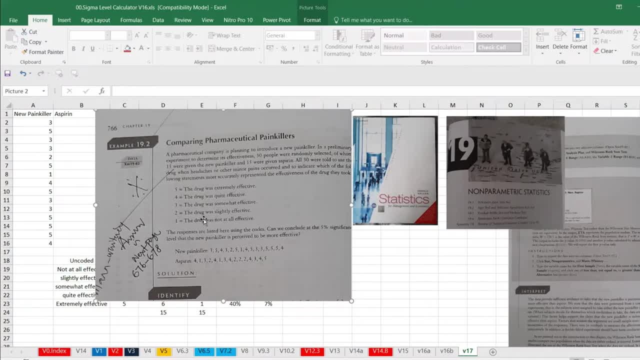 effective. And then this is the for example with three you can just relate somewhat effective. Another person has said it: Five, that means it is extremely effective, and so on, The 15 people you know they've been given with the new painkiller. 15 people has been given with the aspirin. 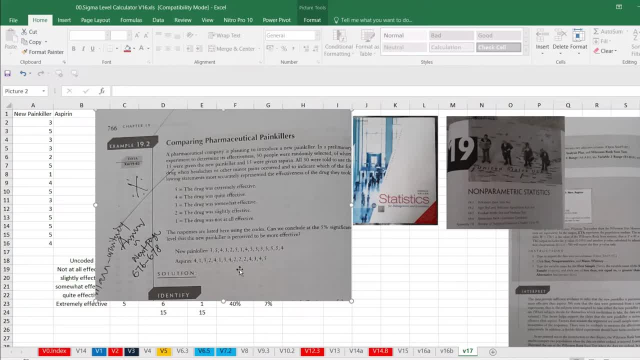 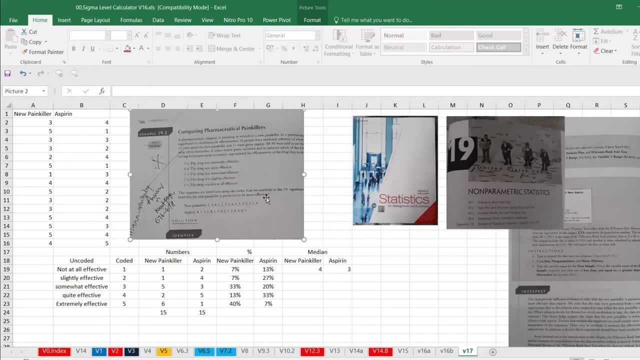 So this is the uncoded. We call them, call them and this is coded. and then so, in this case, non-parametric is something which does not have a parametric right. for example, in this case, you know this will be distribution free. you will not. you will not find any distribution as such right, the histogram or the normal. 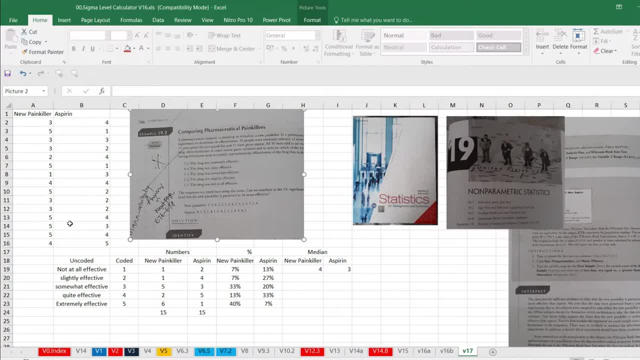 distribution as such. so this fill: in such cases you can go for non-parametric test. so what i have done- basic precursor point directly. you can do it in many tab. but what i have done is so this is the data and i have used count. if formula, and then i counted, that means one not at all effective. 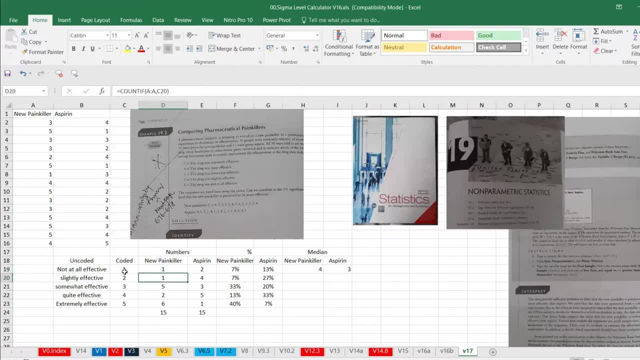 have said one and new painkiller and slightly effective, said one and somewhat effective- five people have said it and quite effective two and then six people have said extremely effective. similarly number, we can talk about the number aspirin one- i mean one, that means not at all effective. two people have said 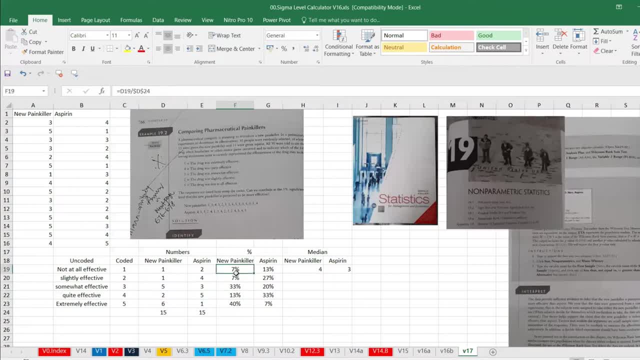 it, and then five people have said quite effective and so on, and this is in terms of percentages, to give you the feel that actually, why we need to do this distribution. can we, can we not conclude that you know this is better and you, you have a forty percent extremely effective. this is better than this, and why not? 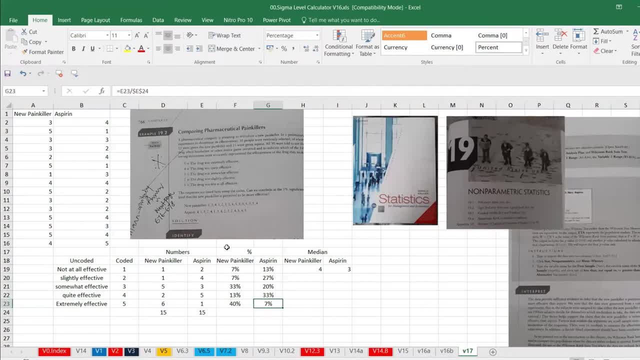 uh, you know, compare this one, so always remember that. i mean whenever you have this one. so this does not follow any distribution. you can't, you can't. for example, the best number we have is 40.. here, the best number we have 33, right 40, meaning like it's extremely effective. that's a good news. 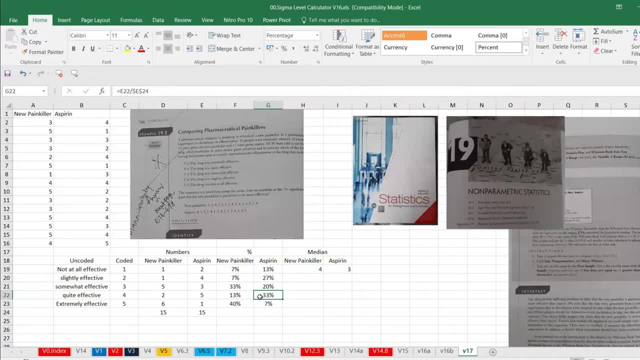 and here, uh four, that is 33 percentage, quite effective. we can't conclude that. that's the reason we need some of the technique, like some of the non-parametric tests, like manwhitney or wilcoxon and all that right. so now the same thing, so this median whenever we talk about non-parametric 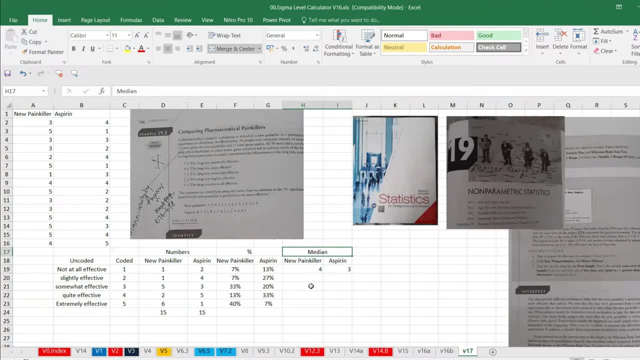 test. it is always: uh, we need to take a look on median. so median is four. that means, in this case, most of the things. the mid value is four. that's extremely good new painkiller. and it's spring is three. that means somewhat effective right. so now what we need to do is- i'm just copying- 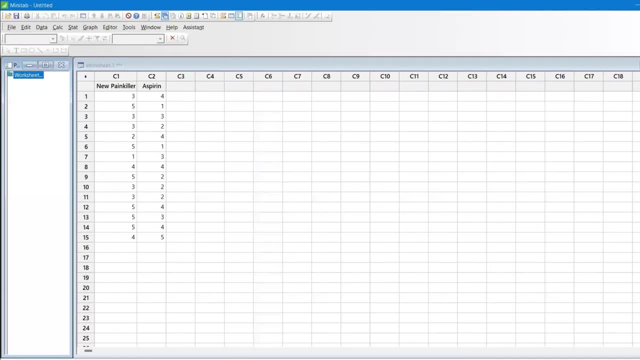 all these value and in the mini tab. so this is the in the mini tab. it has been pasted and you can go to start. you can go to non-parametric test and first thing what we are going to do is manually and determine whether the median of the two group right differs when. 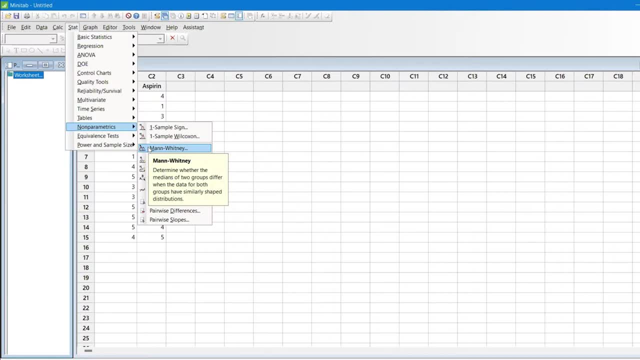 the data for both groups have similarly shaped distribution, similarly ship, like the scale you see, one to five, and there also in aspirin and the painkiller, this the scale is same five, right? so in such cases we can use main whitney, same main whitney if you opposite side, if 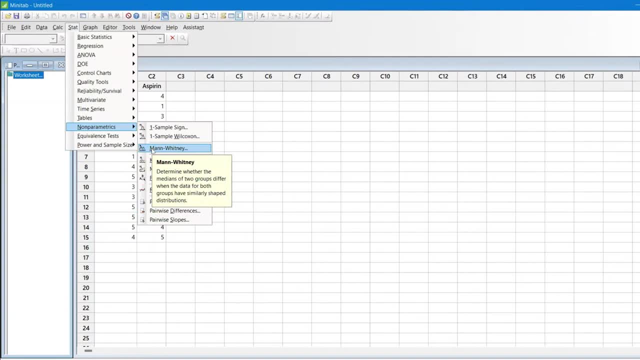 you have a distribution you can use like distribution or continuous data or variable data. you can use two sample t-test, right, but here we cannot do two sample t-test. why? because it does not follow the normal distribution, right. so it has that, the discrete data and with the classification and all that we cannot do. 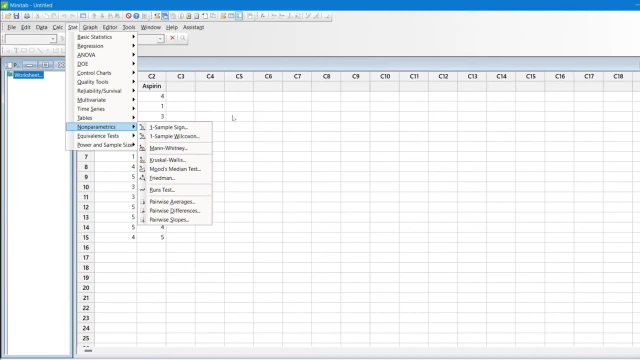 and not only that, we cannot also do a non two proportion test. why we cannot do two proportion test, although it is a discrete but we will not be able to do? because in the two proportion only we need a two category, for example. let me show you, it will show an error. let me show you two. 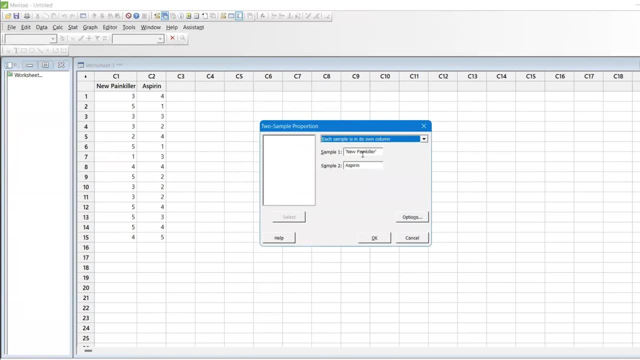 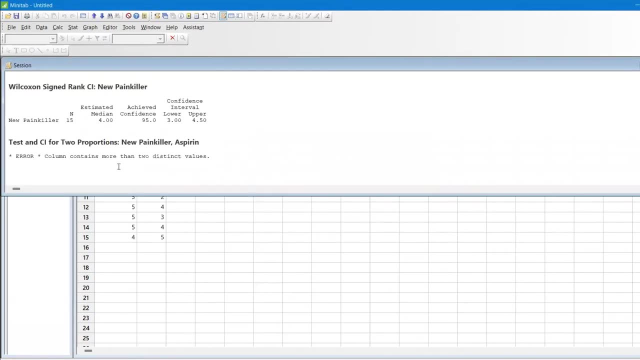 two proportion one. and let's say i have taken a sample one and a new painkiller sample to us and spring it will show us error. right column contains more than two. we need a column should have contain more than two distinct value, so it should have only two value. 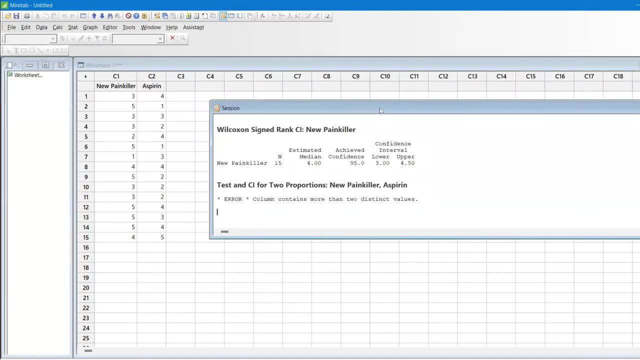 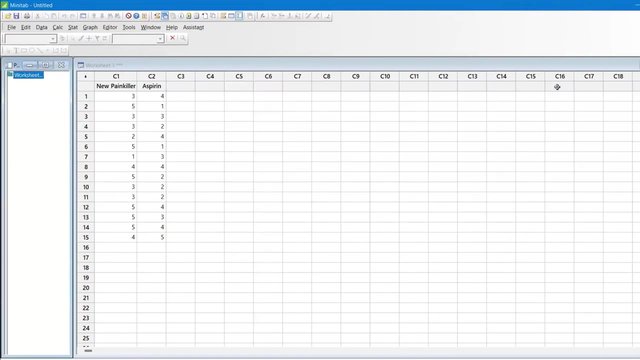 right, like one, two, maybe. one could be, uh yes, and no two could be, uh, other things, right, so r01, r12 or something like that, right? so in this case we cannot use two proportion also as well. uh, the only is, we can only use some of the non-parametric right, so we can take a non-parametric and go to. 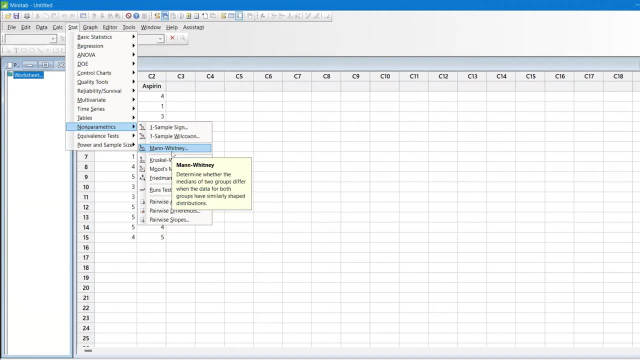 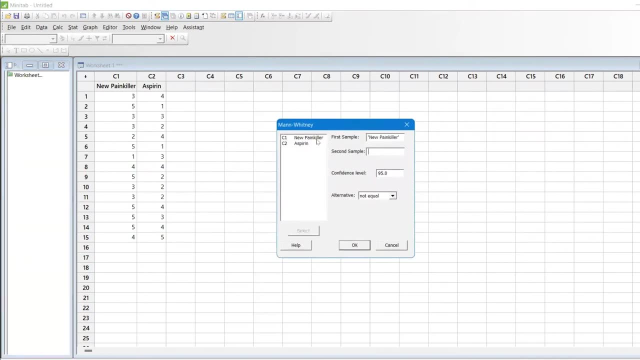 manually, because we are talking about two, uh, two groups, right, uh, whether they are deferred or not. so just have a go and i'm giving the f3. first sample is painkiller, the second sample aspirin and confidence level. we can keep it like 95 in some cases, even if you want 99, you, you can do it. 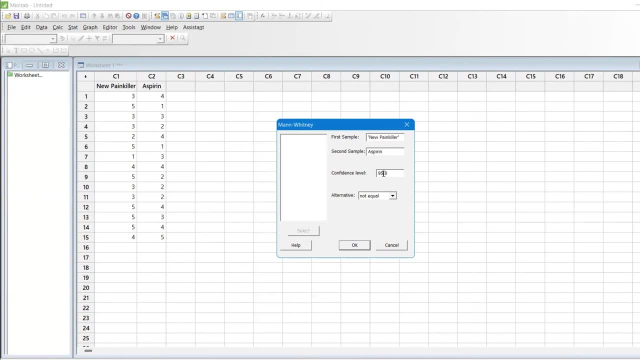 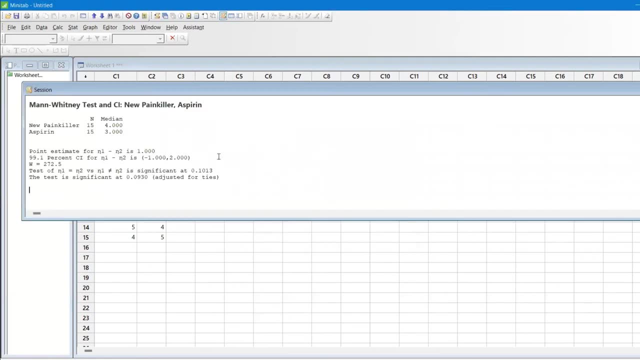 right and this is medicine you don't want to. you want your confidence level to be high. you can do it right. 99 also, you can do it, no problem. so here in this case- uh, you can see, new painkiller is four, median is four, the same thing we got in. 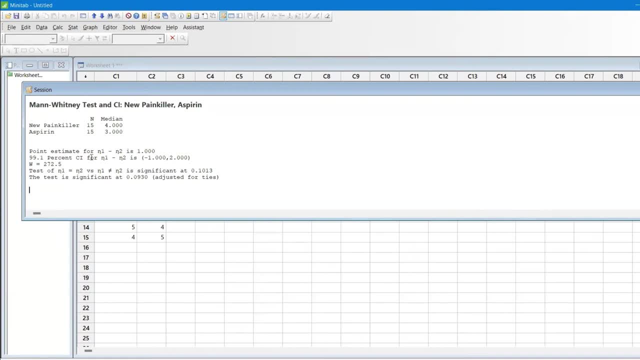 excel aspirin is three and the point estimate for n one minus n two, that is one that before minus three is one and and then so ninety percent confidence it can be uh minus one to two and uh w this main whitney value is 272. that is actually a ranking value and you see, here, uh the test for n. 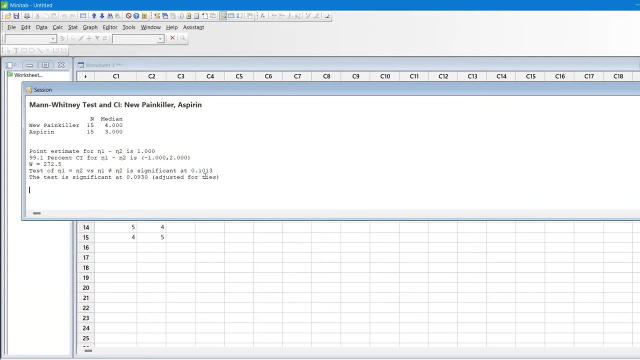 one and n two. so in at this: significant at point one, zero, right, and similarly you can, the test is significant as point zero nine. so the same thing what i will do. i will just keep it like 95 also as well. right so 95, it also says the same value. right, so median we got, and then you.